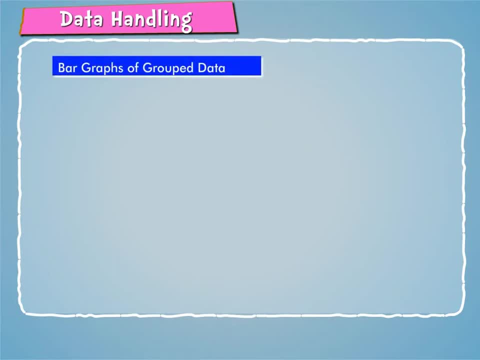 Bar graphs of grouped data. We have already learnt to draw bar graphs of ungrouped data. In this section, we will learn to draw and interpret the bar graphs of grouped data. The bar graphs of grouped data are graphs with no spacing between the bars, For example, 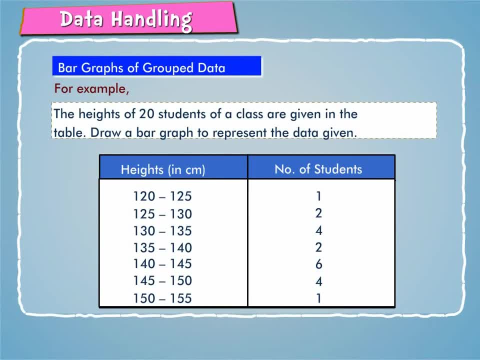 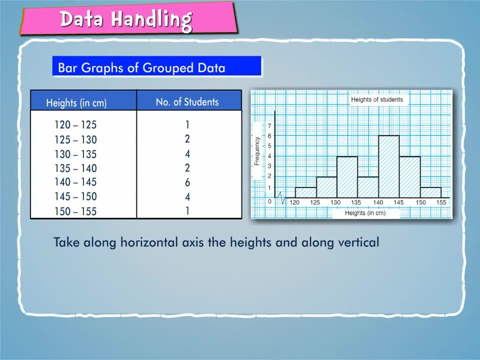 the heights of 20 students of a class are given in the table shown on screen. For this, take along horizontal axis the heights and along vertical axis the frequencies. We represent each class interval by 10 small divisions along horizontal axis and take heights proportional. 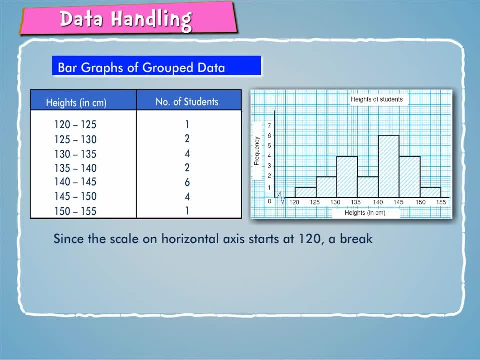 to the corresponding frequencies. Since the scale on horizontal axis starts at 120, a break is indicated near the origin to show that the graph is drawn to scale Beginning from 120 and not from the origin. 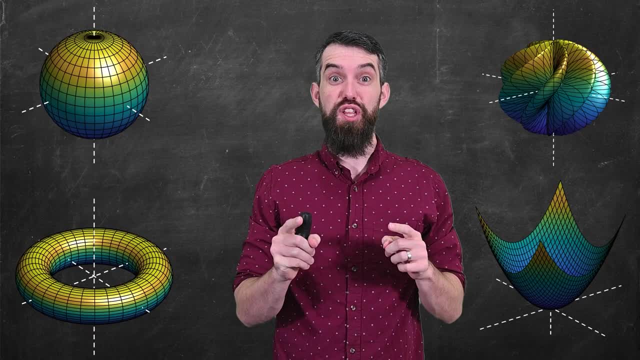 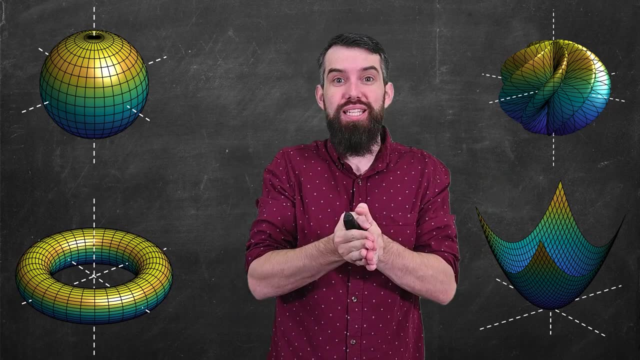 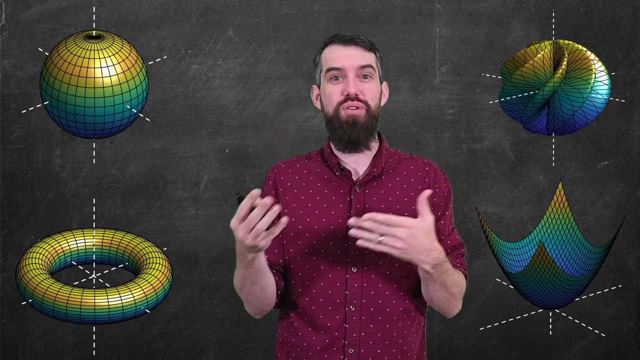 In this video we're going to talk about surfaces like these ones. We're going to try to describe them mathematically in implicit, explicit and, perhaps most importantly, parametric forms. Now this video is part of my whole series on vector calculus. The link to that is down. 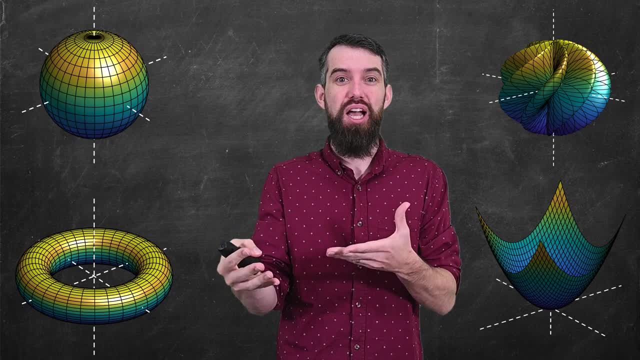 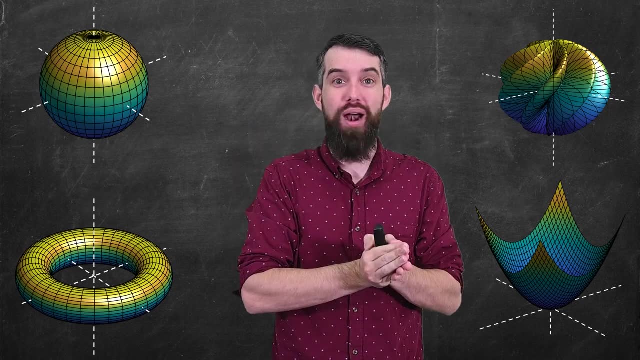 in the description And in future videos. we're going to talk about things like: what is the surface area of a surface, What is the surface integral, analogous to the line integral, as we've seen before, And we're going to ask the question of: well, what would 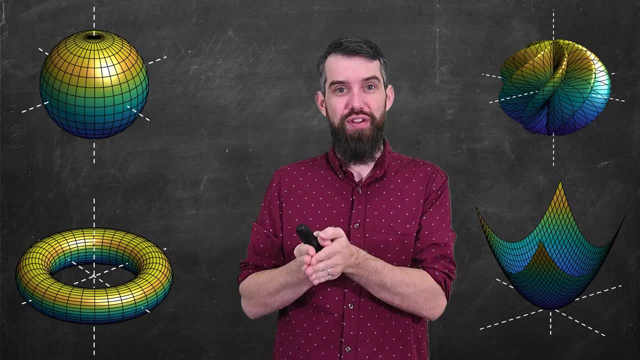 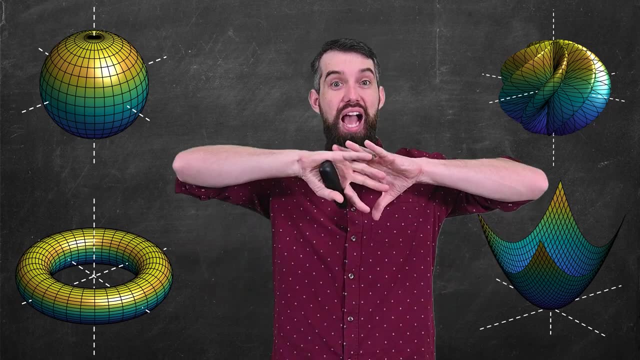 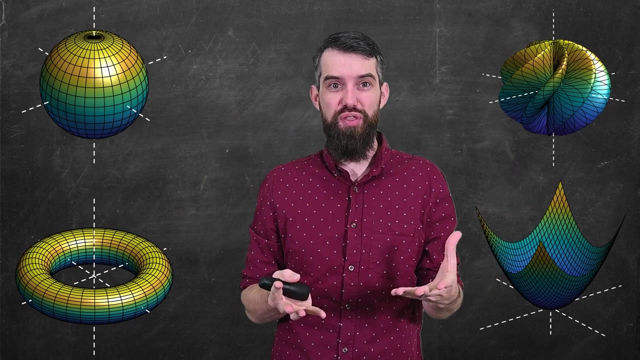 I do if I have a vector field combined with a surface, But in this video we're just going to describe them mathematically. Now, to be clear, I'm only talking about the outside of these regions. I'm not imagining any interior, That is, I'm sort of imagining like it's just the surface of the earth, and